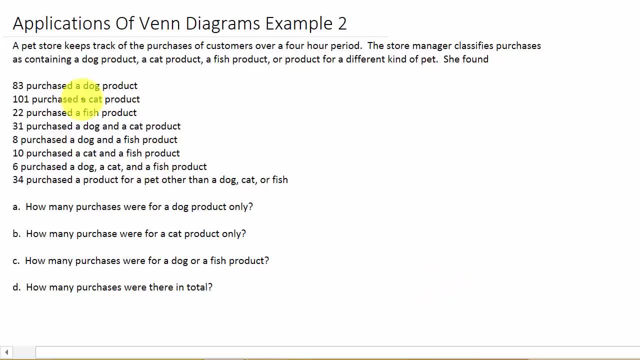 I'll have a link in the description for that. So let's get started on this one. It says here: a pet store keeps track of the purchases of customers over a four hour period. The store manager classifies purchases as containing a dog product, a cat product, a fish product or product for a different kind of pet. She found- and I'm not going to read through all those, but you know she found the number of purchases for a dog, a cat, a fish, a dog and a fish. 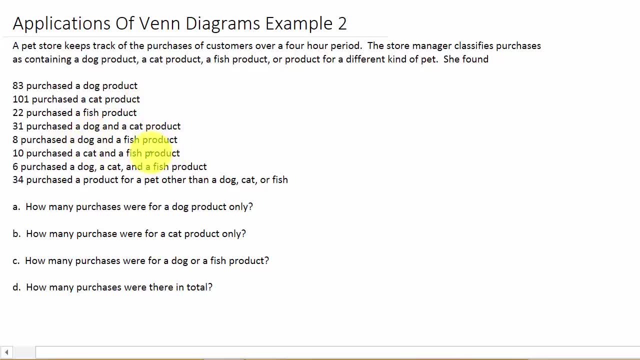 So let's go ahead and let's draw our box and do our Venn diagram. I hope you can read the writing. I know I had to do it kind of small so I could get it all on here. Alright, so let's draw our box and do our Venn diagram. 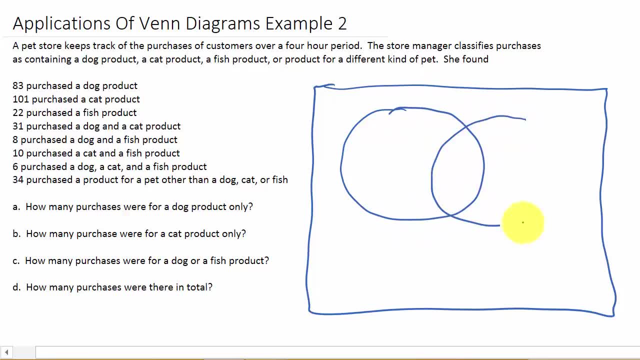 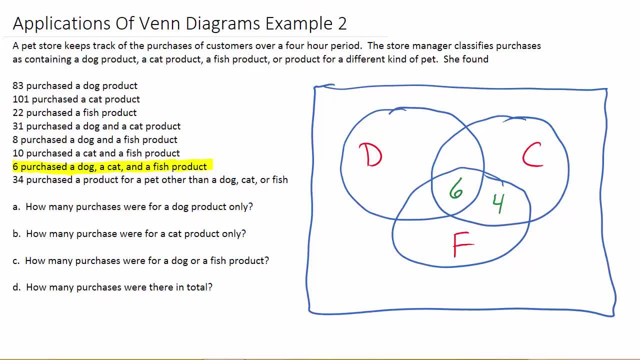 Alright, so let's draw our box and do our Venn diagram. Alright, so let's draw our box and do our Venn diagram, Alright. so here's six of them that already purchased for a dog and a fish, and they just so happened to purchase for a cat also, but we're looking at just the dog and fish right now. 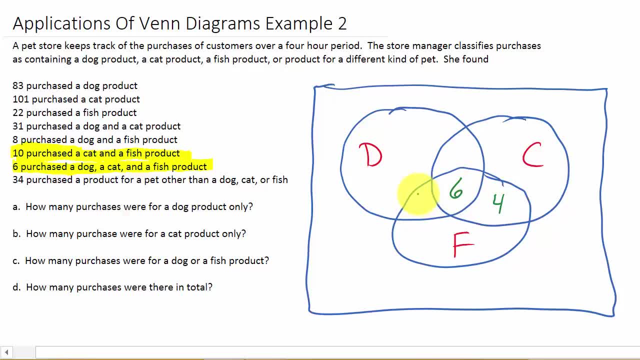 So six plus what Plus two will give me the eight, Alright. so now we've got this one done. Alright. so now it says 31 purchased a dog- Alright. so here's the 31.. See this area, here is a dog and a cat, and it was 31.. 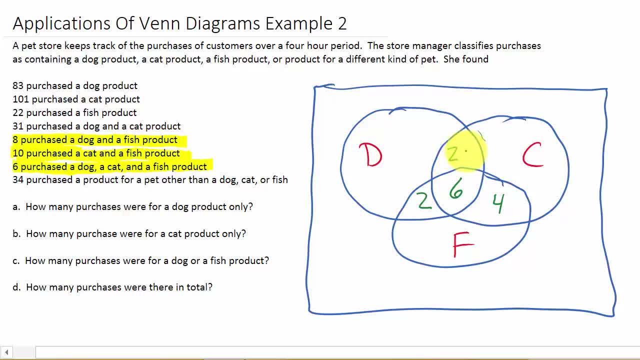 So six plus what 25 is going to total this out to the 31 here. Alright, so this one's good, Alright. now it says 22 purchased a cat fish product. well, you see, the fish product is this whole circle here. so it was 22 total purchased a. 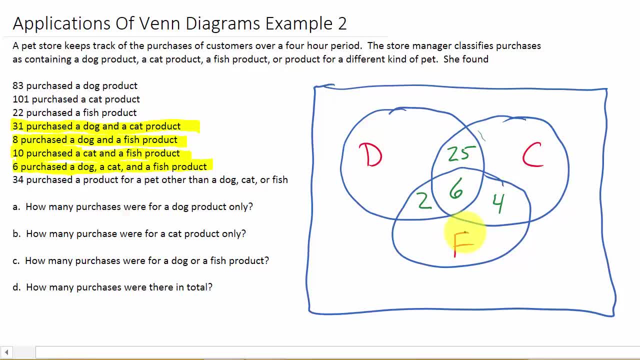 fish product. so if we do 22 minus 4 minus 6 minus 2, okay, 22 minus 4 minus 6 minus 2 and that's going to give me 10, okay. so how did I know that this right here should not have been 22 instead of 10? 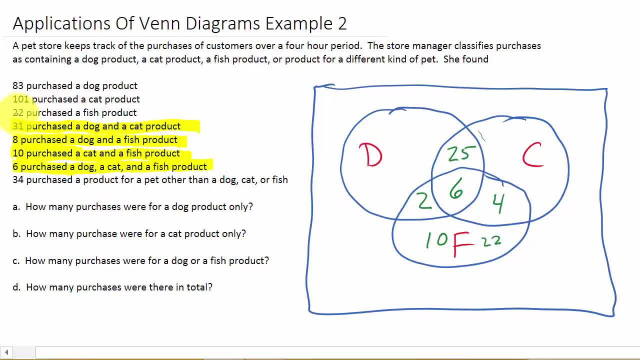 okay, because it did not say 22 purchased a fish product. only now, if this would have had only on the end of it, then it would have been 22, but it said 22 purchased a fish product. so the 2 plus 6 plus 4 plus 10, that's going to total the 22 for the fish okay. 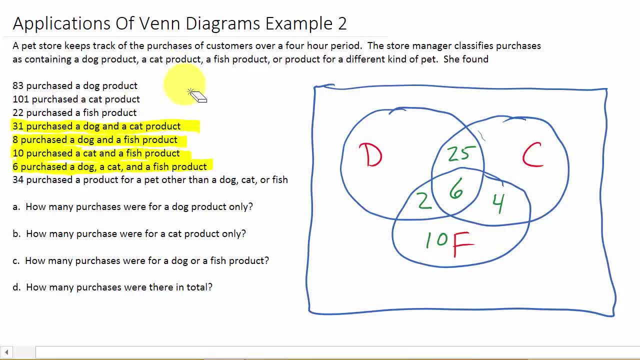 all right, so now we have the fish product done and then a hundred and one purchased a cat product. okay, so here's the cat product right here. okay, so to get what goes here, all of these numbers in the circle for cat have to total to 101. so we'll do 101 minus the. 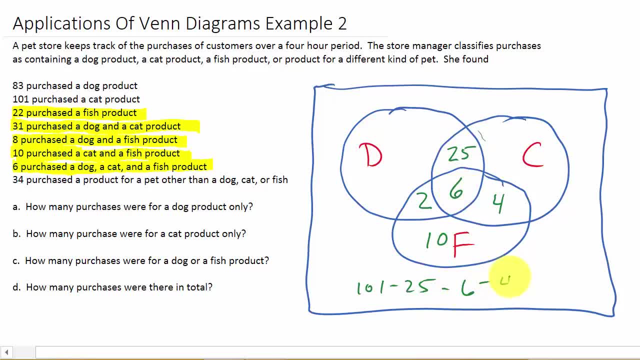 25 minus the 6, minus this 4, and so I've got 101 minus 25 minus 6 minus 4, and that's going to give me 66 here. okay, all right. so now this one's good, and now we have 83. purchased a dog. 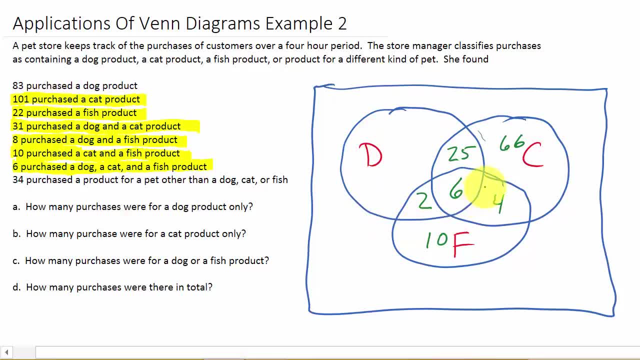 product. so that means this circle here for the dog. this has to total 83, okay. so what goes here? well, that's 83 minus twenty five minus six minus two, and so eighty three minus 25 minus 6 minus 2 is 50. all right, so we're done with this one. and then it says: 34 purchased a. 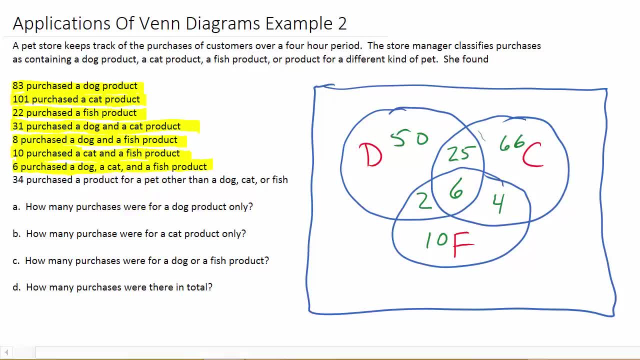 product for a pet other than a dog, cat or fish, so that would be purchased for an animal other than these three. so that would be outside of the circles. so that would be 34 out here. all this space outside the circles represents other pets. okay, all right, so now we can answer our questions. 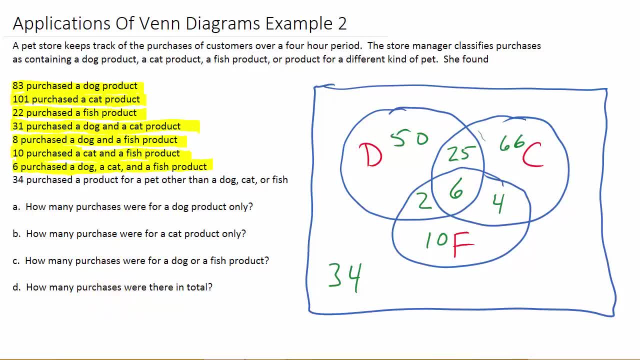 all right, so now it's easy to answer the questions. so it says how many purchases were for a dog product only. okay, so you can see there's 83 total for a dog. but they're wanting to know purchased for a dog only see this: purchased for a dog and a cat, this purchased for a dog, cat and fish and these two. 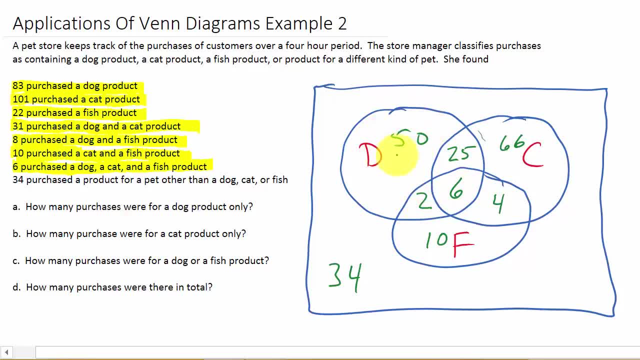 here purchased for a dog and a fish. well, the 50 here purchased for a dog only. so that answer would be 50.. and then how many purchase purchases were for a cat only? well, that would be the 66 here. and then how many purchase purchases were for a dog or a fish product? a dog or a fish? so hopefully. 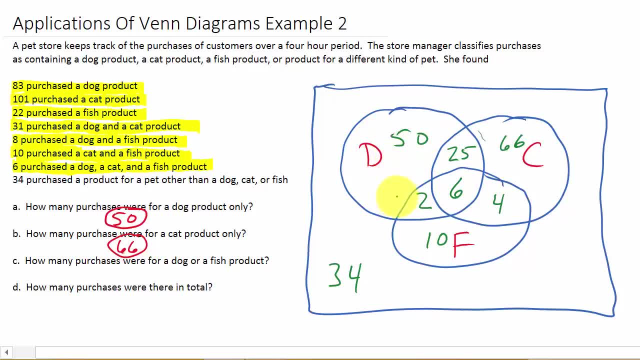 you can see this, that's everywhere. there's a number for a dog and a fish. so i'm gonna, i'm gonna hola them so we can keep up with them, so we can see here this 50, the 25, here the 6, the 2, the 4 and 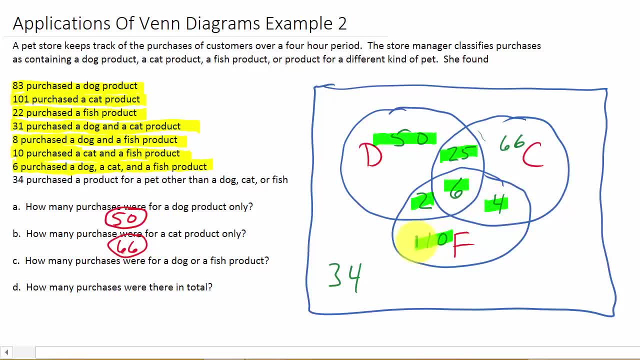 the 10. okay, all right. so how many purchases were for a dog or a fish product? and so everything that's in the dog or fish circle is going to be counted. now what if it said how many purchases were for a dog or a fish product only? well, that would be just the two here. see that, alright. so 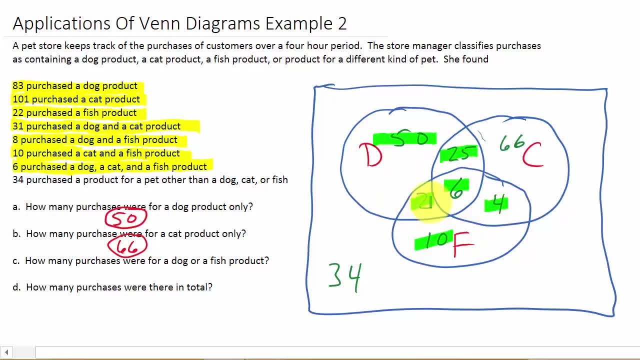 what we have to do is add all these numbers up, and so let's see what we've got. we got 50 plus 25 plus 6 plus 2 plus 10 plus 4 and add all those up and that would be 97. that's adding all these numbers up that are: